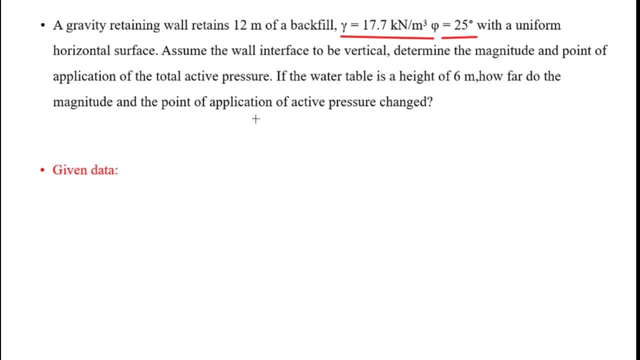 height of 6 meter, how far do the magnitude and point of application of active pressure will change? so basically, we'll start with the given data. height is given, 12 meter, gamma and Phi are given. important thing which is not given is the value of C interface to be vertical over here. if you can see somewhere over here it is. 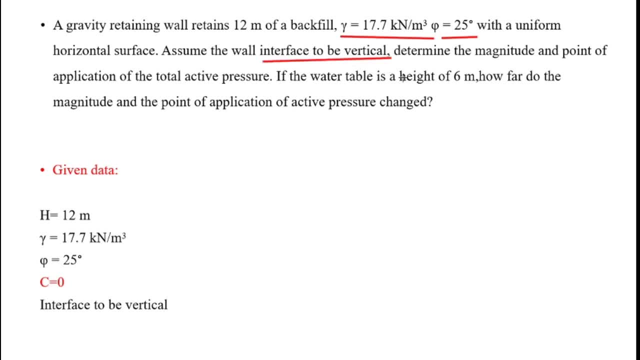 given interface to be vertical. this is a very important thing in deciding what kind of method do we need to solve this miracle. okay, what else is given? friction angle is not given. again an important thing. the friction angle between wall, wall and this backfield soil is not given. so these three things, see wall interface and 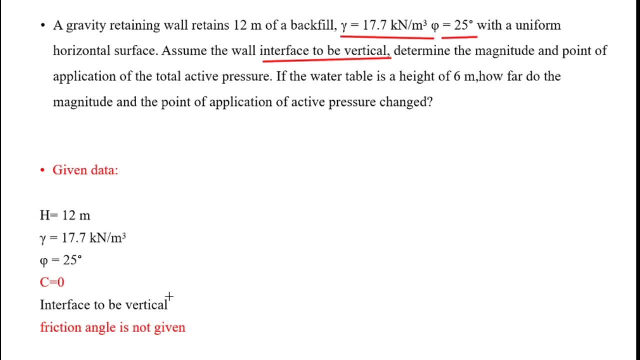 friction angle help us decide which type of method is to be used. so what does it say? it says that Rankine's method is to be used. okay, next thing is: if you look at carefully, read this numerical, you will realize that this numerical is basically divided in two different. 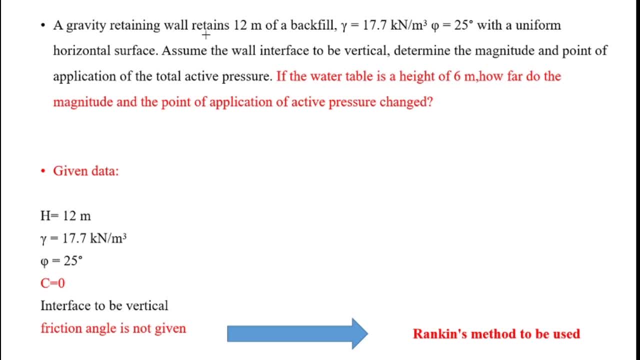 part, the part one that you see over here which is in black and the part two is in red. okay, so in part one you can see over here, I have divided into two cases. the case one: no water. case two: water at six meter from the top. if you want to represent these two cases into a diagram, 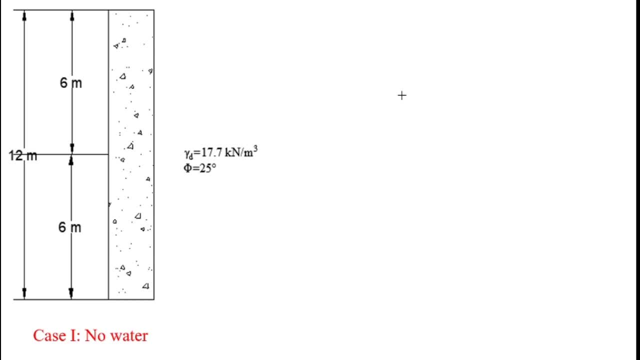 of format you can see over here. this is your part one: there is no water. so when there is no water, whatever the value of gamma is given, it will be gamma dry and in case two, a water table at a height of six meter is given. now, because of that, what happened? the soil above the water table is a 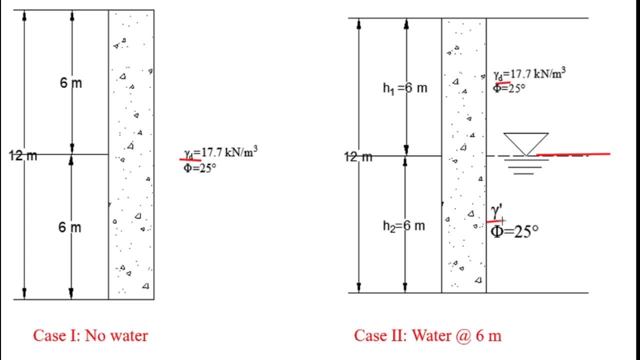 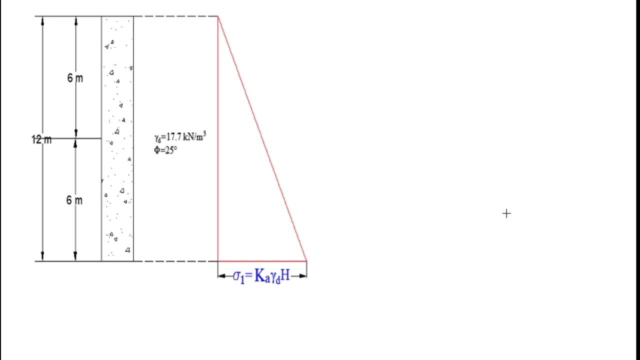 dry soil in the soil below the water table is a submerged soil. that's why I have used different symbols over here. at the top I have used gamma dash- sorry, gamma d- and at the bottom I have used gamma dash. okay, so what we'll do? we'll start with case one, wait a second, okay. so case one is very simple. 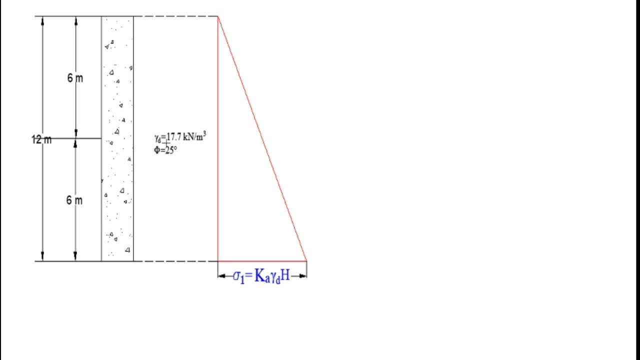 entire soil is a uniform with a gamma equals to gamma d equals to 17.7. so first we'll determine this stress distribution diagram. stress distribution is fairly simple, so this is for case one. sigma one equals to k, gamma d into h. so that will be your stress distribution diagram and 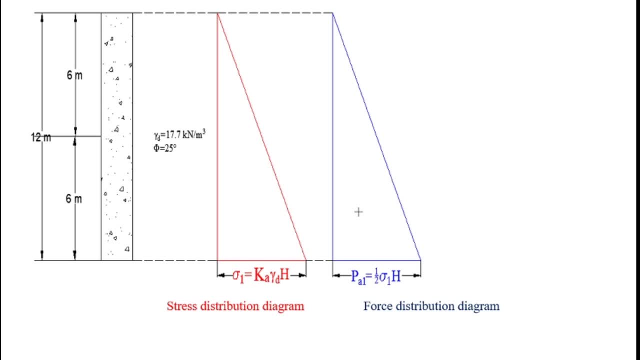 next is force distribution diagram, which is in blue as we are discussing. the class force distribution diagram is nothing but area of stress distribution diagram. so if you want to determine, if you determine area of this diagram in red, you will get this blue diagram. okay. so how do you determine? area of triangle is nothing but base. 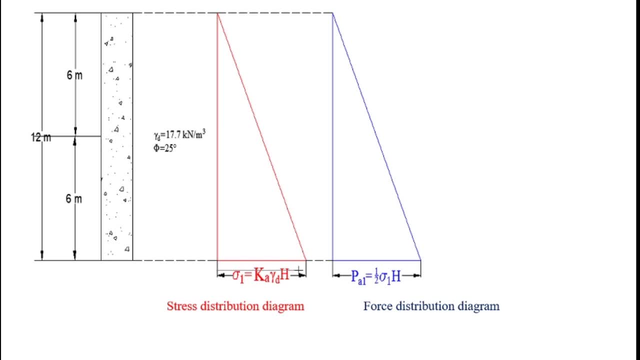 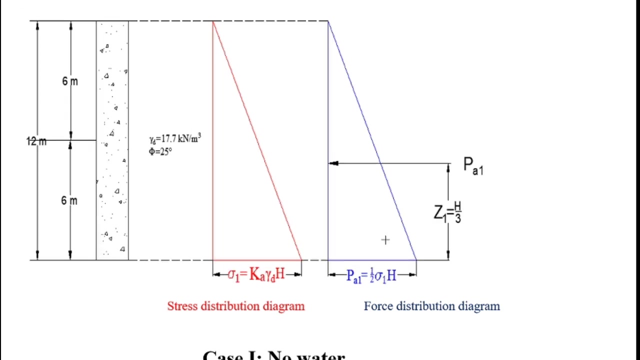 half base into height. so this is your base, that is sigma one, and this entire height is your h. okay, so area becomes half base into height. so this is how you get force distribution diagram and stress distribution diagram. next step, what we'll do? we'll determine the location of this force, pa. this is the pa one that we have determined. 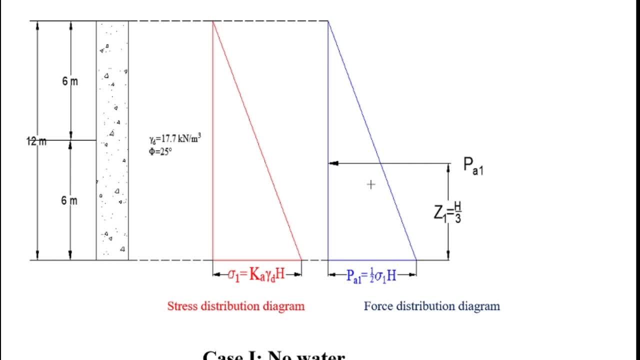 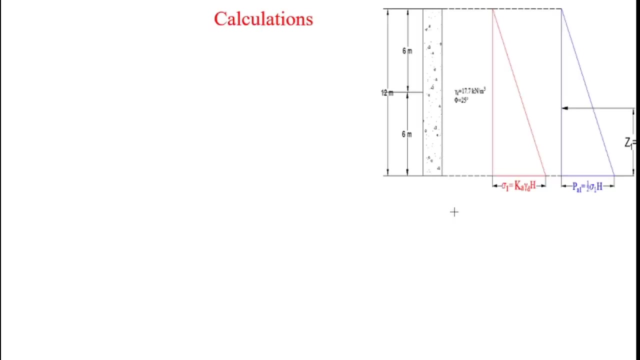 over here, as there is only one diagram. as I have told you earlier, this will be fairly simple, numerical. so you have only one diagram. so pa one act at height z, one which is equals to h by three. now the calculation part is very simple. first of all, we'll determine the value of k. 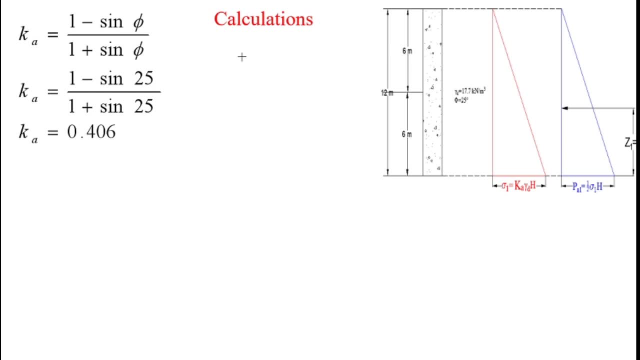 it's a Rankine's method and the search is very simple. so we'll determine the value of k. we'll determine that the surcharge is horizontal, as there is no search charge over here. so k equals to one minus sign five divided by one plus sign five, you get a value of k equals to point for zero six. similarly you will get that value of sigma one, which is k gamma D, into Edge at that value as eighty six point two. next we'll determine pa one. pa one equals to half sigma one into edge and that value comes as a five one seven point two kilo Newton Holz. and we'll determine Pa1- PANO- I have a U error- and that value comes ten times as a AmannN flexor, also known as a penuon square. The parameter comes again in a positive. sigma1 Lw comes as a copy of sigma1 and pa-1 are created in below. the solution of sigma one becomes an equality here. so here is that: two k, twice plus the value on the odd square and sum table. and simply remember over and over again: this is the phi one, their Bridges to self. 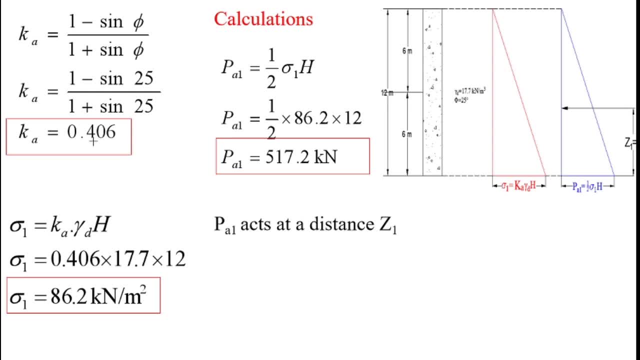 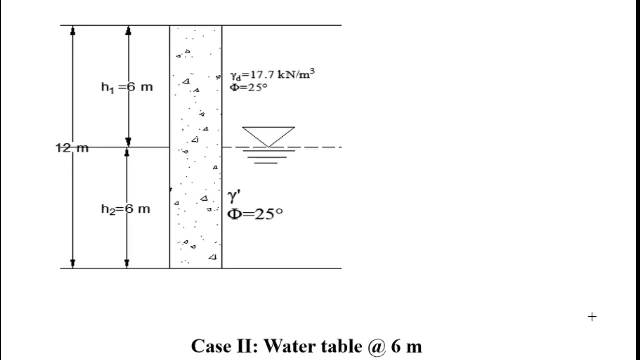 and don't forget the units. next, PA 1 acted a distance z1, so z1 equals to h by 3, which comes as a 4 meters. as there are no other forces, this, your PA 1, becomes your resultant, that is, equals to PA. next we'll go with the case 2. in case 2, what is happening? there is a water table. so you have. 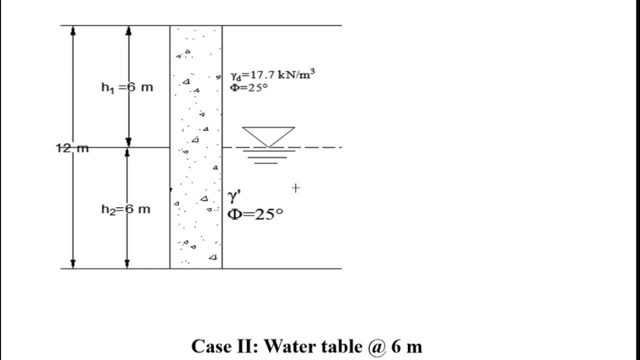 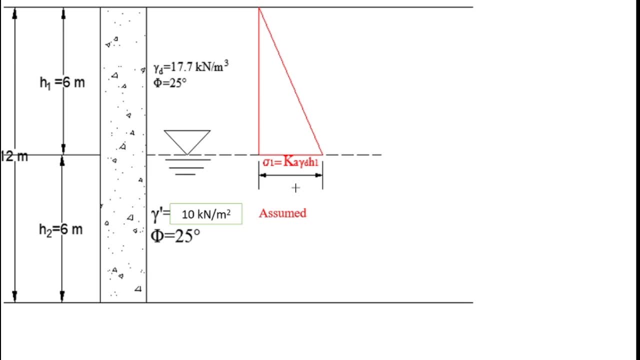 this soil is nothing but a submerged soil. okay, so first we'll determine stress distribution diagram, and before that there is an important thing that you need to keep in mind: the value of gamma dash is not given. there is a formula for determining gamma dash which is equals to gamma dash equals. 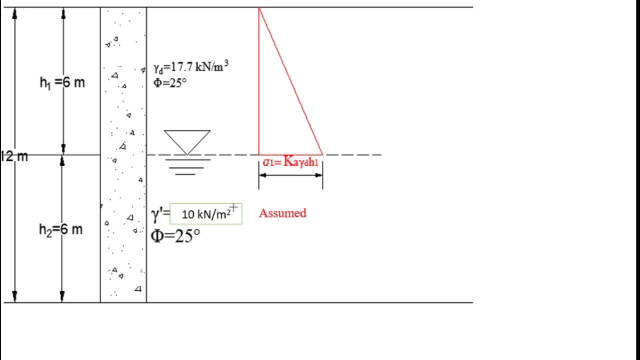 to gamma submerged minus gamma w. but we cannot use that formula as the value of gamma submerged is also not given. so whatever done over here, I have just assumed the value of gamma dash as a 10 kilo Newton per meter square. okay, so we'll start with the stress distribution diagram. stress distribution diagram for this soil. 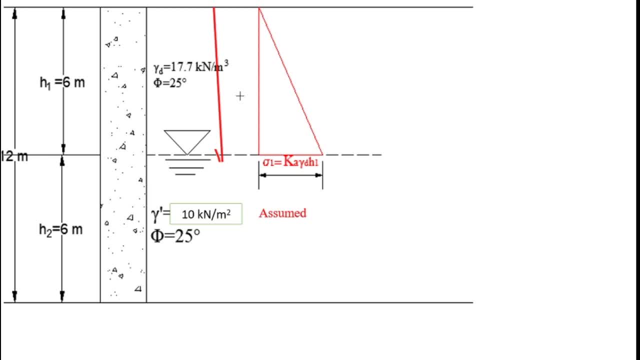 from top till this point is this one, that is, Sigma 1, which is equals to K, gamma D, into h1. h1 is nothing but over here 6 meters. okay, the Sigma 1 will come down this. let's call it as a figure number 1. 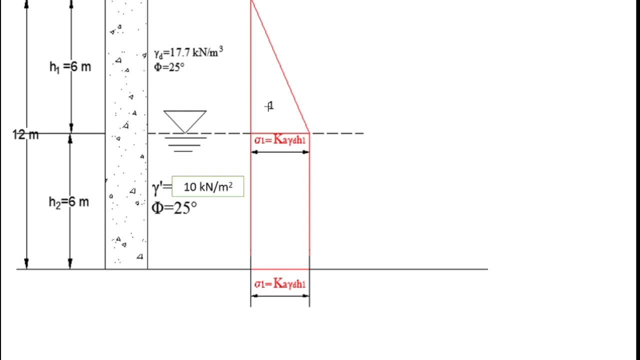 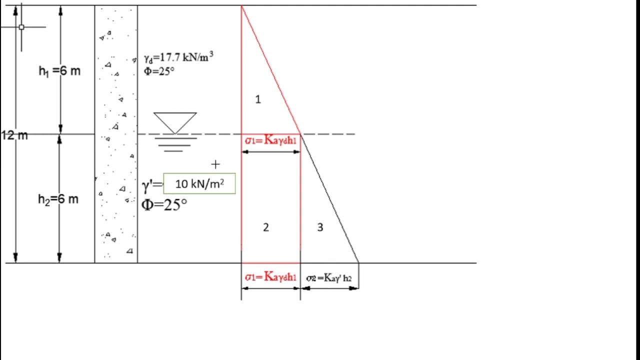 next thing: the Sigma 1 will come down, as it is, till the bottom. let's call it as a figure number 2. then we have figure number 3, which is nothing but the stress Sigma 2, due to this submerged soil over here, the submerged soil that you see. gamma dash because of that. because of that you get K gamma. 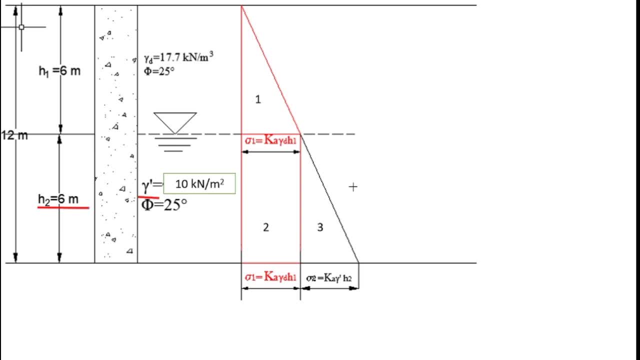 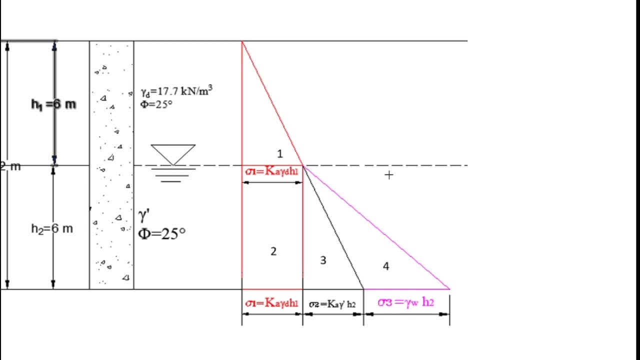 dash into h2. so this is your h2 6 meters. okay. and the fourth, and the important one, is the diagram number 4, which is due to the water which is present over here. whatever this soil is there, this soil contains water and because of that water there. 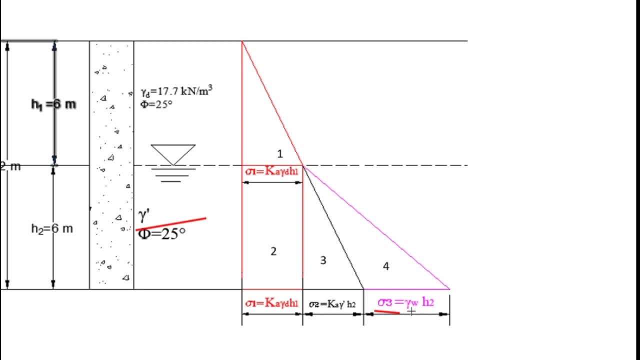 is this Sigma 3 which is coming. an important thing to notice, Sigma 3, is that you don't have K over here. this is very important. don't make mistakes, any mistakes over here. we have discussed in the class why K doesn't does not come over here. that is because of Pascal's law. I'll not go into. 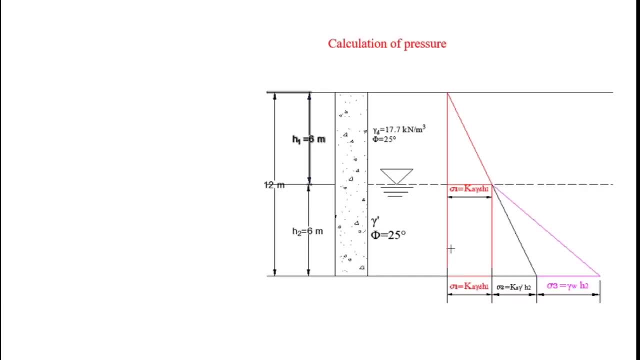 the detail over here. okay, this is next thing, what we'll do, all these forces, all these stresses. we are determined. we'll just do the calculation. as Sigma 1 equals to K gamma d, h1, that value comes as 43.1. similarly, you get a value of Sigma 2, K gamma dash h2, that value comes as a 24.36. Sigma 3: 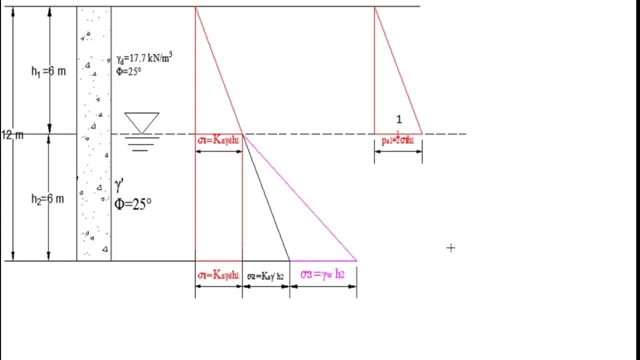 0.86. now next phase will move towards determination of force distribution diagram. force distribution diagram, as discussed earlier, it is nothing but area of this diagram. gives you a this diagram. okay, so now your force distribution diagram. so first, p a1 equals to half of base, that is Sigma 1. 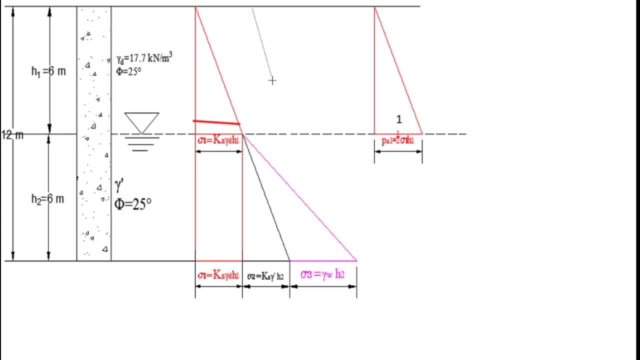 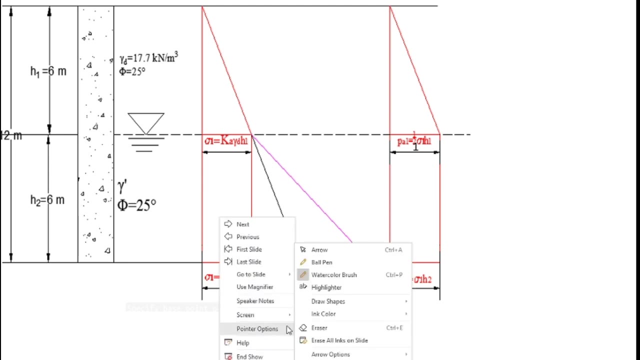 into height. that is 1. so this is your height and this is your base. so it comes as a half: Sigma 1, H, 1. similarly this for this diagram. let me change the cursor, let's take arrow. okay, so for this diagram, you get force distribution diagram over here. it looks like this, as it is a rectangle: the 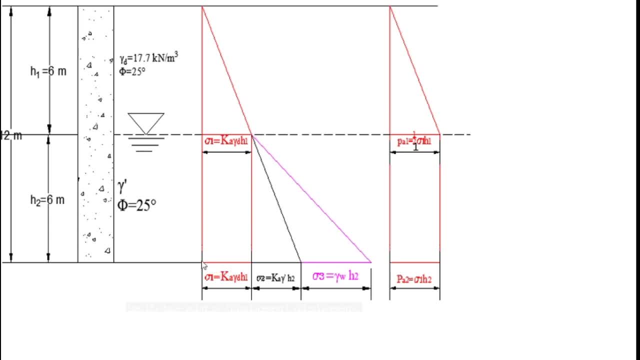 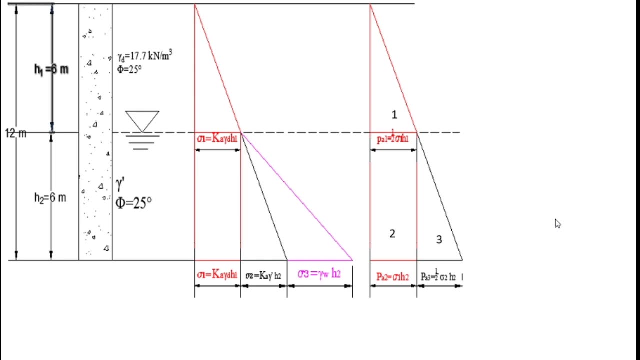 area will be simply this face multiply by this height. okay, it's called it as a figure number 2. the figure number 3 will give us a PA 3. PA 3 will be equals to. it is corresponding to this diagram, so its area will be equal to. this is the base and H 2 is the height. 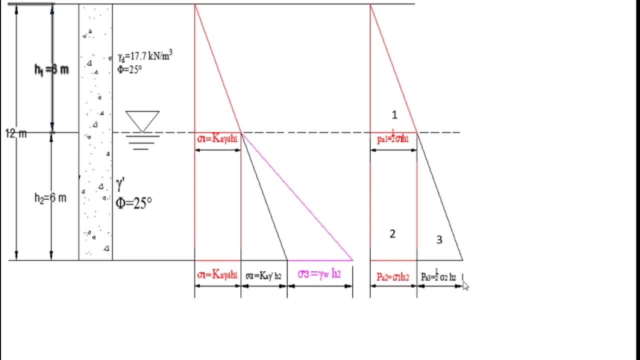 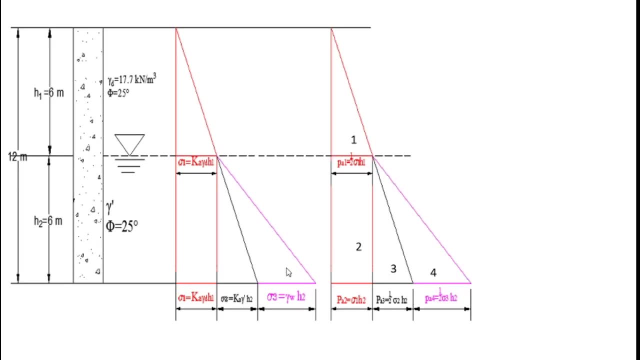 so your PA 3 becomes Sigma 2 into I, sigma 2 into h2. similarly, the fourth diagram comes as the area of this diagram. so the base is sigma 3, height is h2. so your pa4 becomes half of sigma 3 into h2. now let's do the calculation. 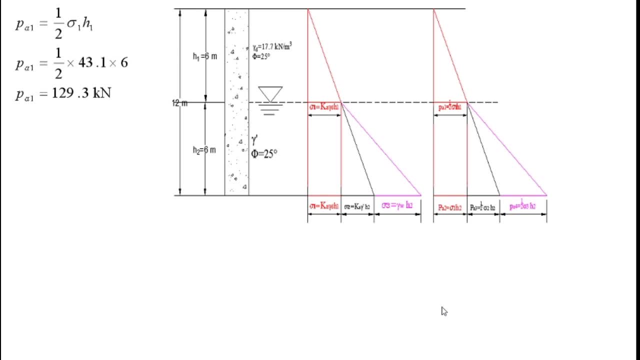 calculations are very simple. once you determine these formulas, the calculation becomes very easy. pa1 equals to half sigma 1, h1. that value comes, as the 129.3 pa2 equals to, as this is a rectangle, sigma 1, into h2 area of rectangle as a base into height. then, similarly, you get a value of pa3 and. 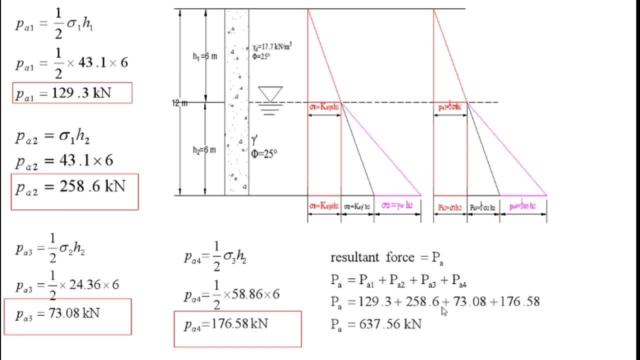 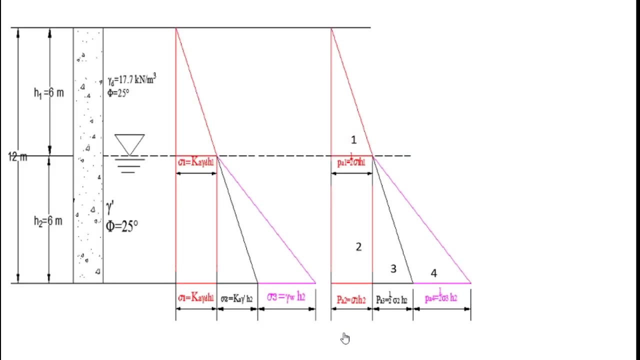 you get a value of pa4. now resultant force pa equals to summation of all individual forces, that is, pa1 plus pa2 up to pa4, and that value comes as 632.56. next important thing is to determine the location of all these individual forces. if you can see over here, your PA 1, your PA 1, will be acting. 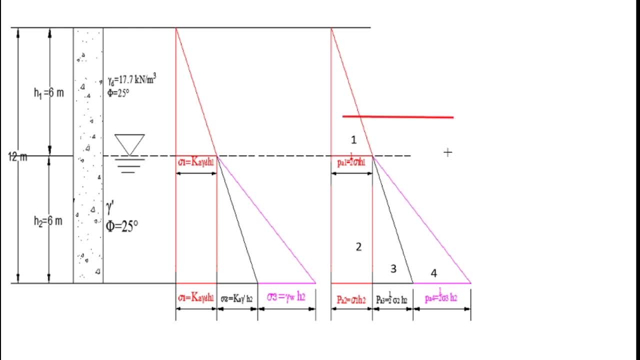 somewhere over here. so PA 1: act at a distance this much from the bottom. how much is this? okay? how much is this distant? the distance equals 2h 1 by 3. okay, this distance is H 1 by 3 plus H 2. so basically, what do you? 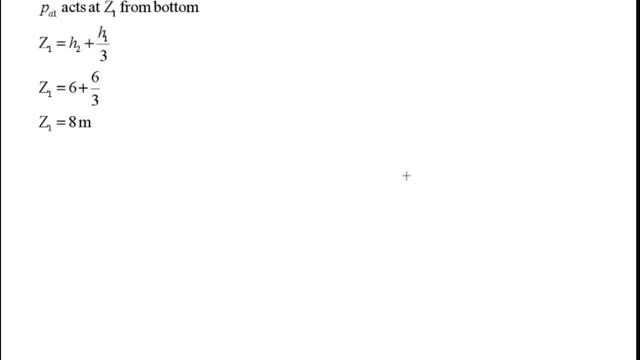 get over here. said: 1 equals 2 z1. PA 1 acted is Z 1. so Z 1 equals 2, H 2 plus H 1 by 3. PA 2 acted a distance Z 2 from the bottom. where is PA 2 located? 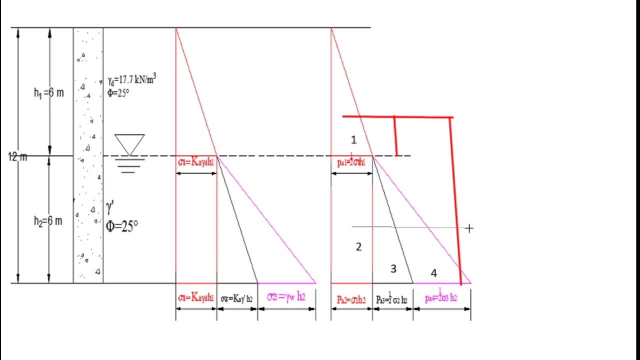 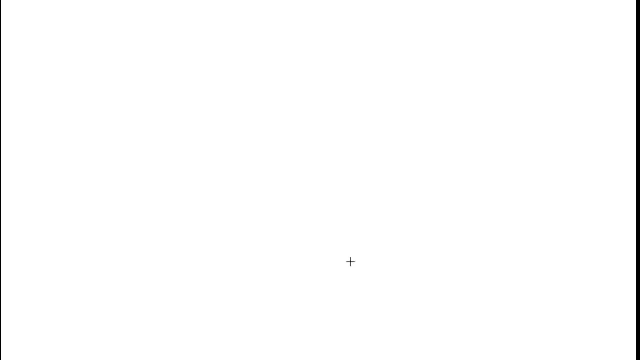 PA2 is located somewhere over here, so PA2 will be acting at a distance. this is for rectangle, so PA2 will be acting at a CG of rectangle, so CG of rectangle is located at H2 by 2, so this distance will become H2 by 2, so that distance H2 by 2 as a 3 meters, similarly PA3. 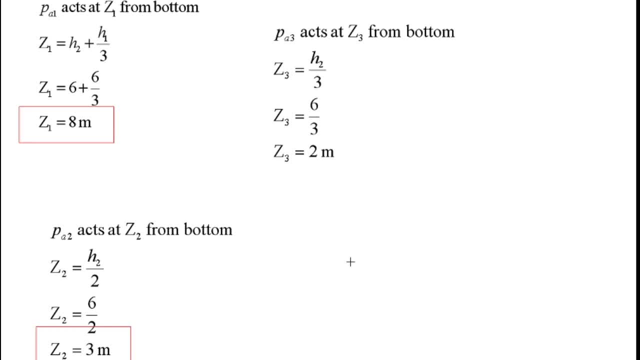 and this is for a triangle, so it will be H2 by 3, PA4 will be again for, PA4 will be acting at a distance, Z4, and Z4 is again for a rectangle, that is for our figure number 4. so let's say: 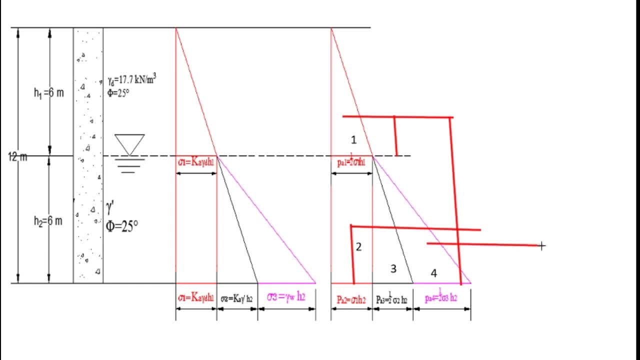 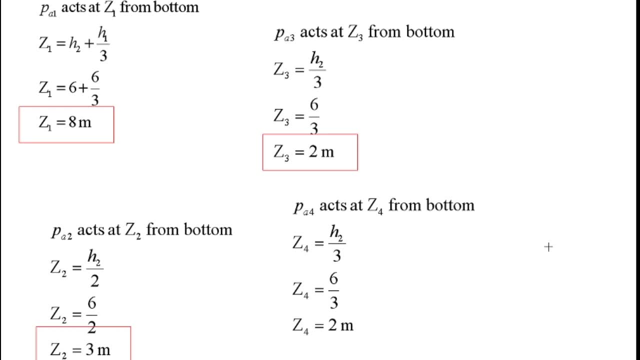 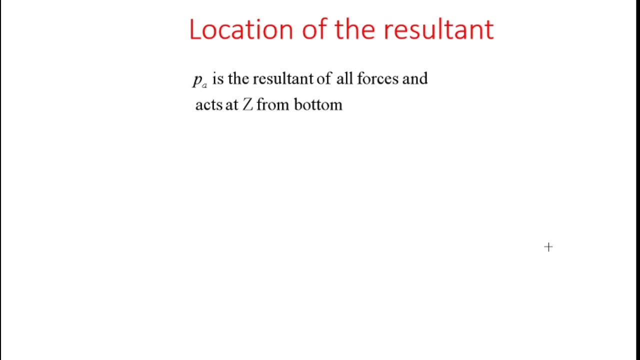 this is your PA4. so this distance is again H2 by 3. so you see over here, H2 by 3. next is location of the resultant. How do we determine location of the resultant? Let's say PA is our resultant, which we have determined. let's say it act as a distance. 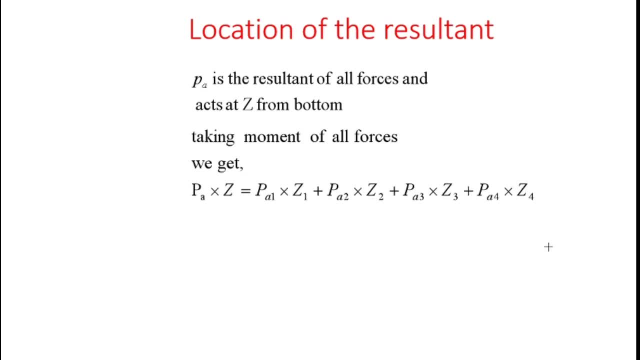 Z from the bottom. so, taking moment at the bottom, you get equation like this: PA into Z equals to PA1 into all individual forces and their distance from the bottom. once you do this and solid for Z, you get the value of Z as a 3.6 meters. okay, now the important. 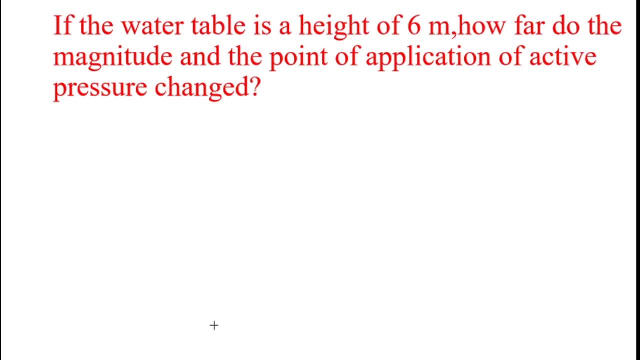 thing. what was asked in the question is In the question is: If the water table is at height of 6 meters, how far do the magnitude and point of application of active earth pressure changes? so he is asking us both the things, magnitude as well as point of application. so first we will see the magnitude, how far the magnitude will change. 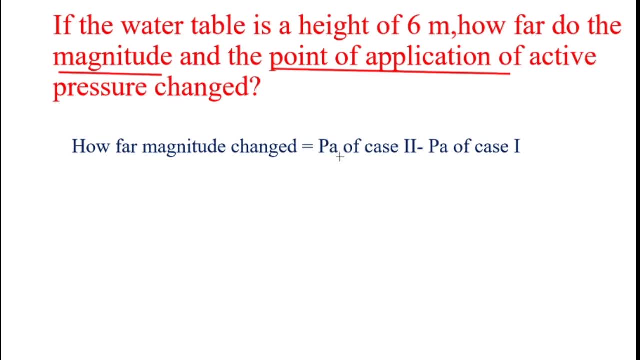 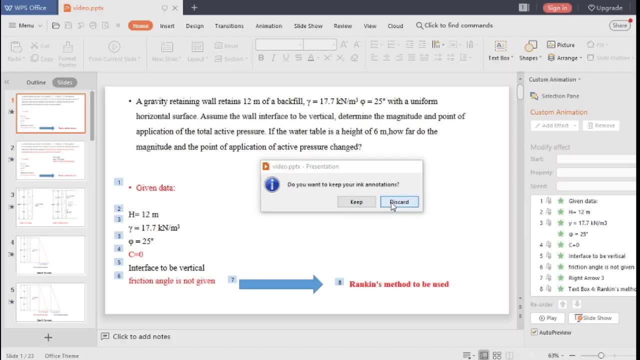 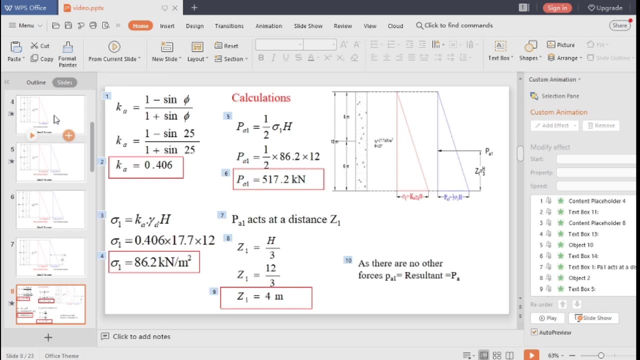 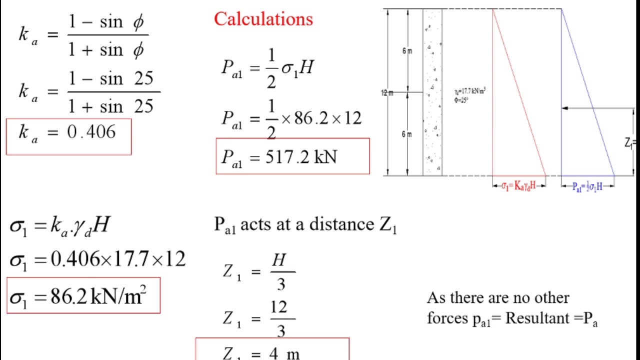 so, basically what we have to do, we have to do PA of case 2 minus PA of case 1. okay, so this was our case number 1. let me discard this, Let's go and let's see, Let's go at the top. so this was your PA over here. so this was your PA of case 1. this was: 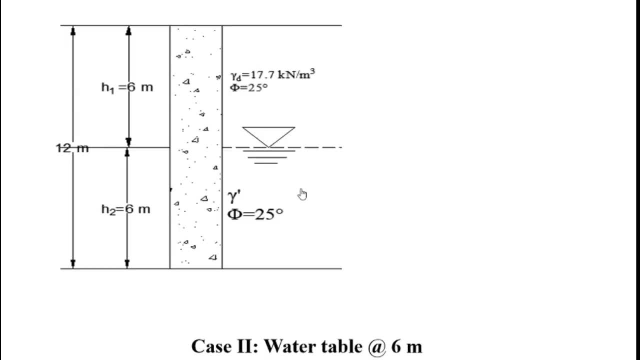 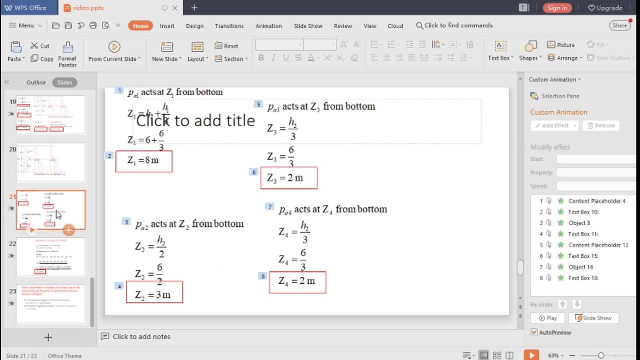 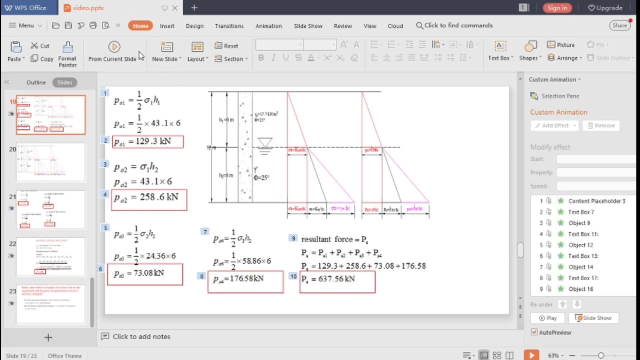 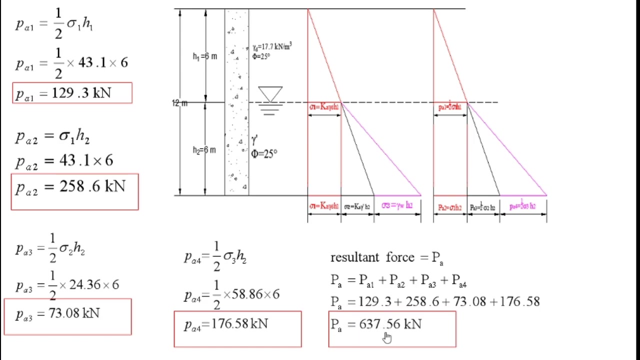 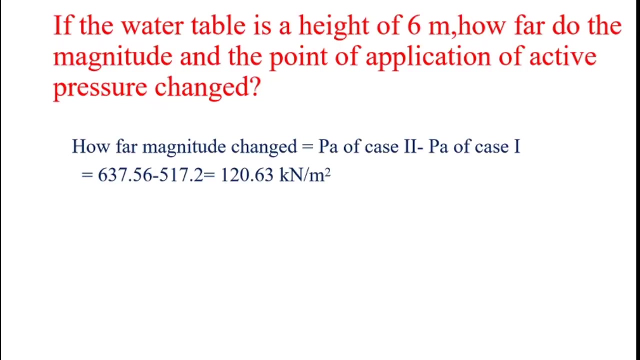 PA of case 1 and PA of case 2. we have just determined over here PA of case 1. where did it go? yeah, this is your PA of. okay, it should not have done that. okay, PA of case 1 is here. so we just subtract these two values, so PA of case 1 minus PA of case 2, you get value. 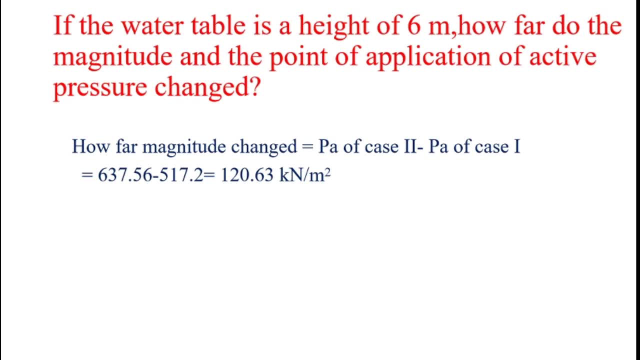 of 120 kilo Newton, 120.36 kilo Newton per meter square. so to the question: how far? okay, Okay, Okay, Okay, Okay. So the magnitude question is solved. next thing is asking us how far the point of application will change. okay, so for that, what you need to do, Z of case 1 minus Z of case 2. now why?